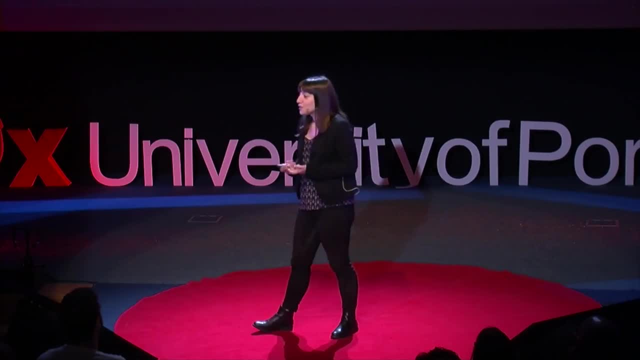 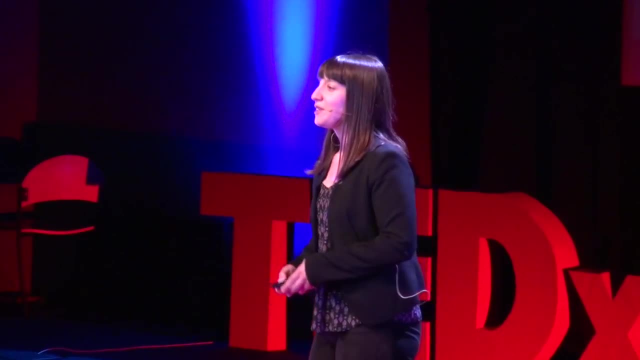 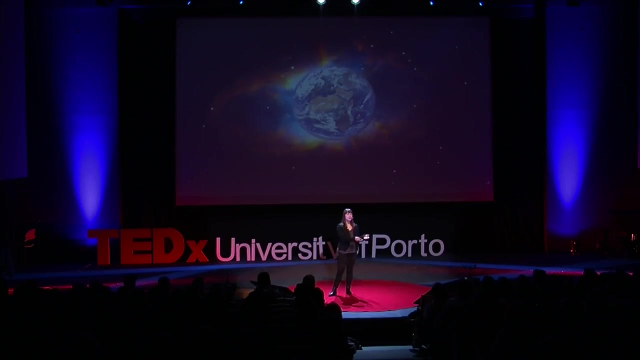 about life, in other words what it could be. the only logical starting point is to start by looking at our own species, planet, right, because for now, the only planet that has life is earth. so what we do is something called the great analogy, and in here we use all the knowledge that we have from life on earth. 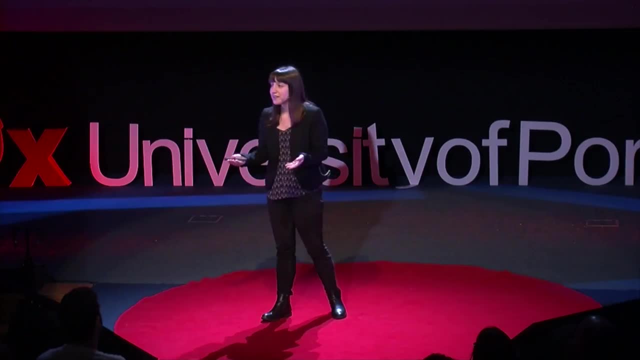 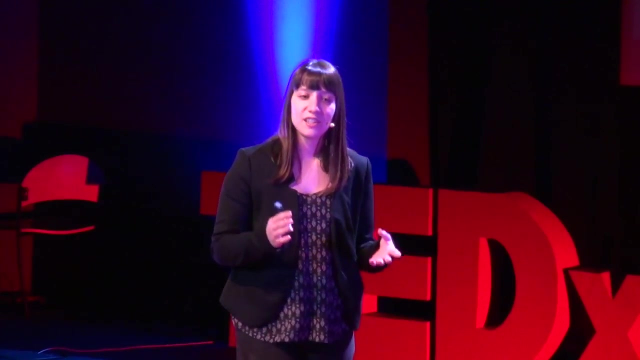 how it originated, how it evolved, what it looks like now, in which environments it lives in, and we extrapolate this knowledge to other environments in the universe, to extraterrestrial environments, to what other places of our solar system and beyond. so the origin of life on earth. 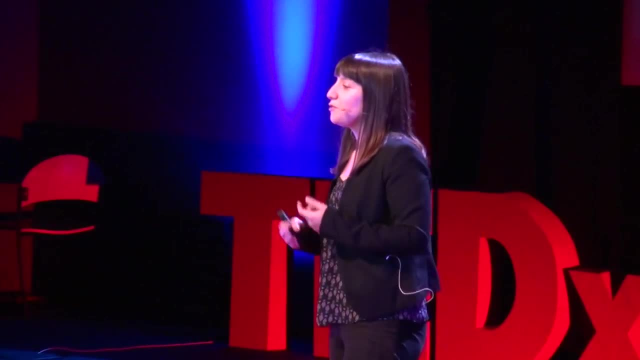 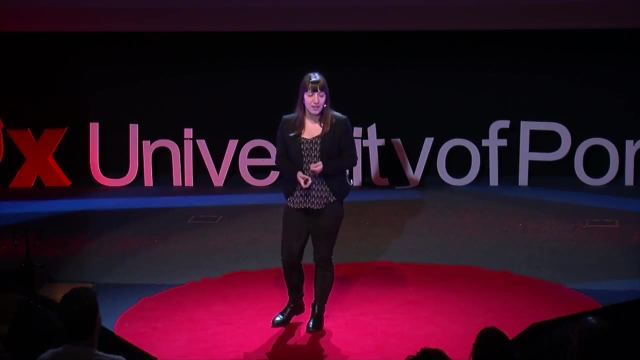 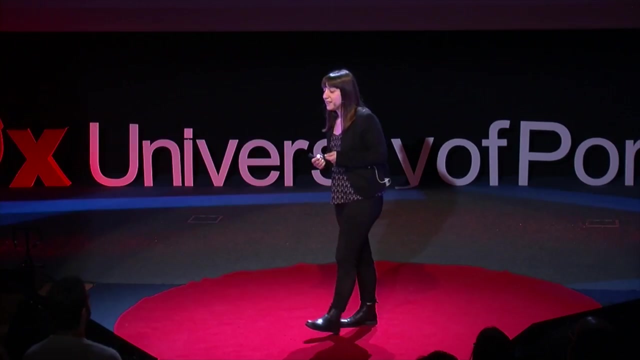 is one of the key main happenings for astrobiology, because if we understand how life began here on earth, then we know what it takes for life to have emerged in other places right. so on earth life is thought to have emerged around 3.8 billion years ago, and back then earth was not the same as today. 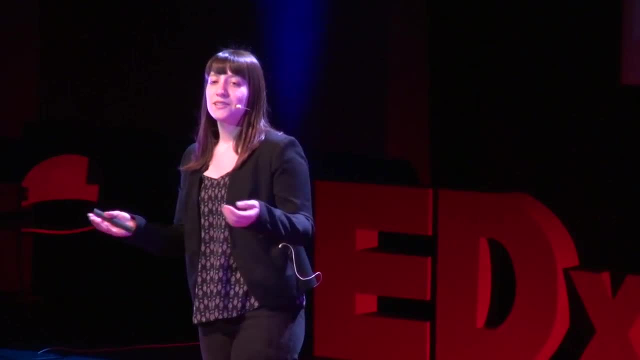 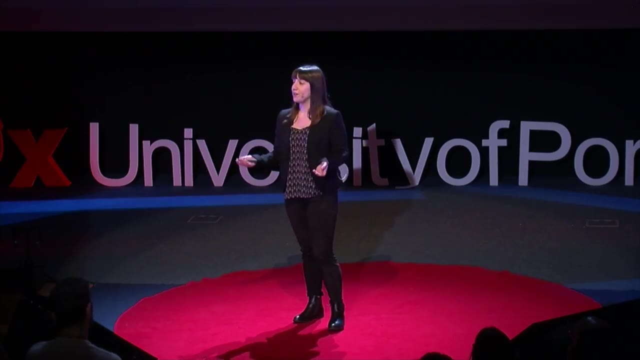 there was no oxygen, the ozone layer wasn't there, so we had a lot of radiation, and so the first forms of life would have to be anaerobic, so they would have to be able to grow up without oxygen and they would have to find a way to protect themselves from themselves, from the radiation. this means that 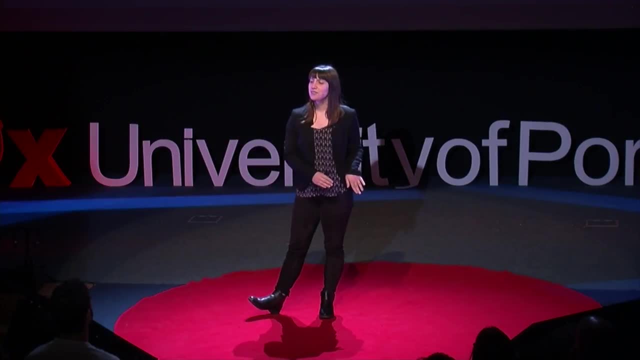 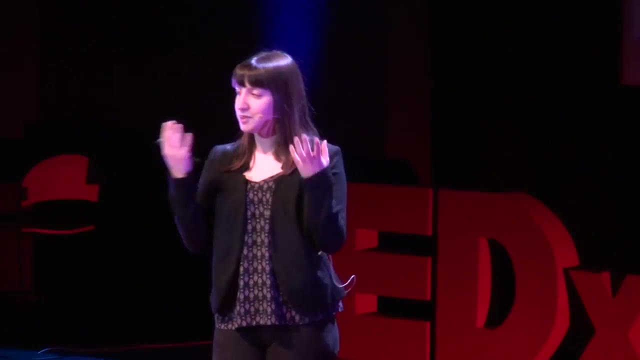 one of the possibilities is that life was, uh, first originated in the deep oceans, where the radiation wouldn't hit. so okay, what it takes for life to emerge, at least as we know now, two things: liquid water, and water and oxygen. that's what we call the level of oxygen, that's what we call in the 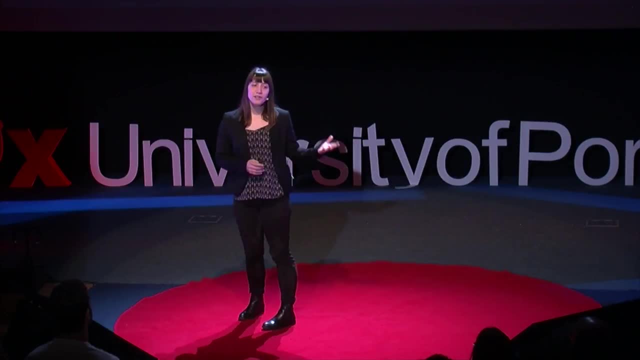 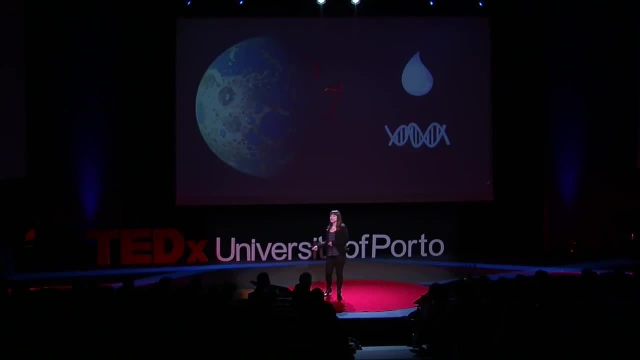 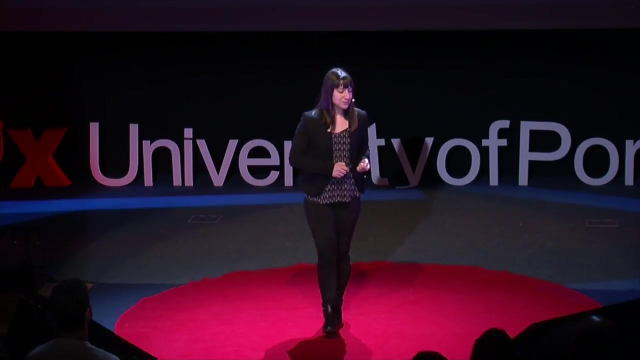 and organic molecules, so on early earth. what we think is that the oceans would bring the molecules around, the tides would bring the molecules around and eventually the right molecules met at the right time at the right place and life emerged. the planet Earth evolved. there are many different life forms now. 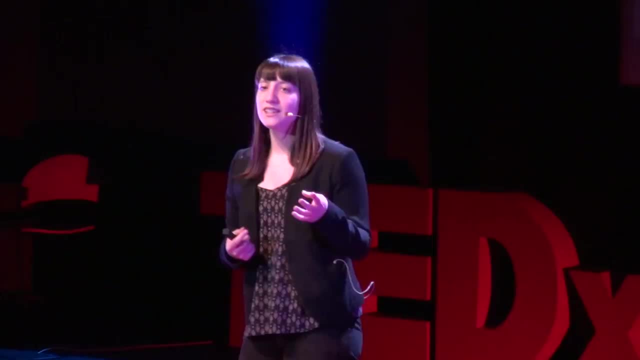 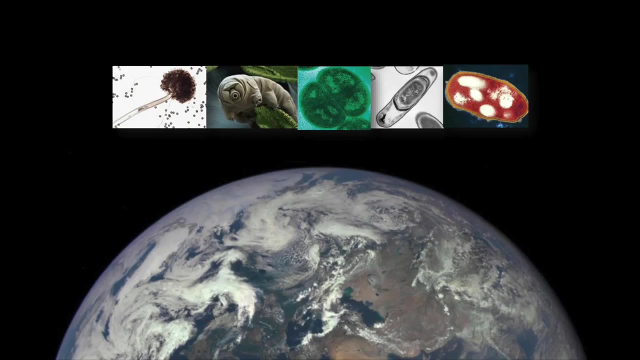 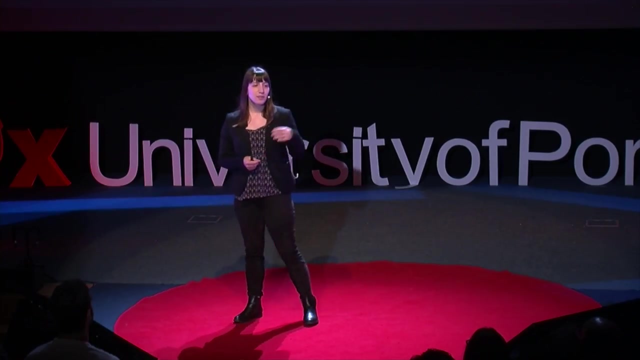 right and biodiversity really is pushing forward, because every day we find new organisms that live in places that we thought no life could ever exist. they are so extreme. these guys are called the extremophiles. these are just some examples of microorganisms that live from temperatures from minus 20 degrees. 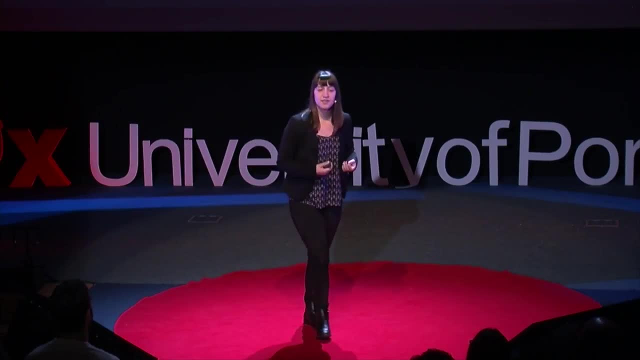 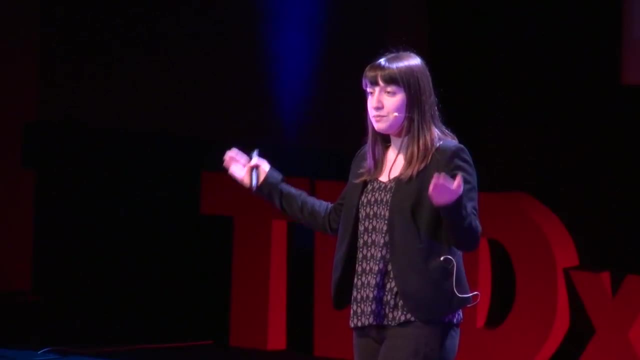 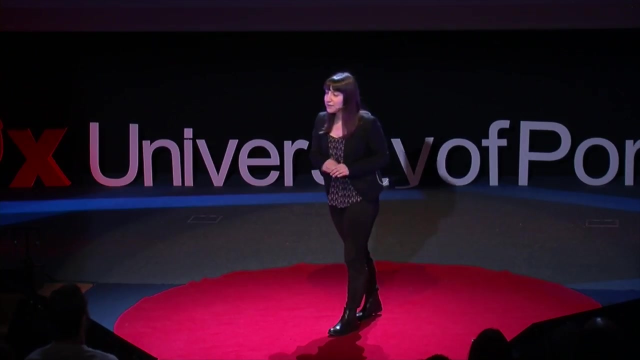 to above a hundred. they live in very acid rivers or very salty lakes, and these extremophiles are essential for astrobiology because they help us set the limits of life. we help, they help us understand in which environments life can actually exist. one of the most extreme environment is actually space. so here on earth we have the ozone layer, as I said, the magnetic field that keep us protected. but once you go up and you leave the ozone layer and you leave the magnetic field, you get hit by the space radiation, solar, cosmic radiation. you get hit by the space vacuum. you get hit, not hit, but you are in microgravity. you would have no. 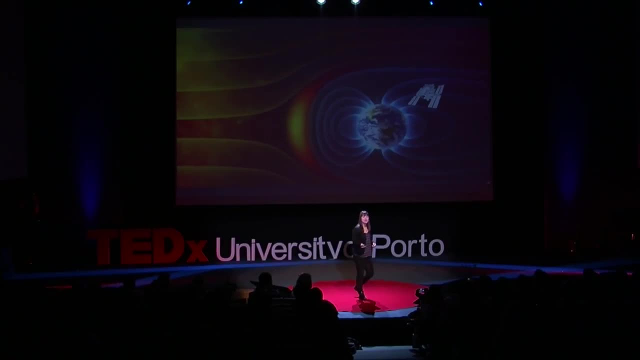 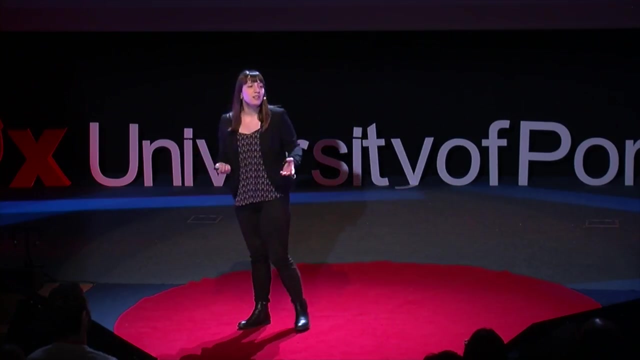 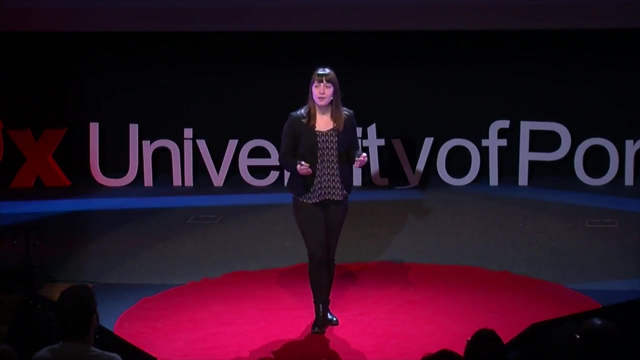 gravity and astronauts that are in the International Space Station they know this very well. temperatures are very difficult to control as well, so one of the things that we want to know is: can Life survive in space? we have been doing a lot of experiments, many of them are simulations, so we have ground-based facilities that 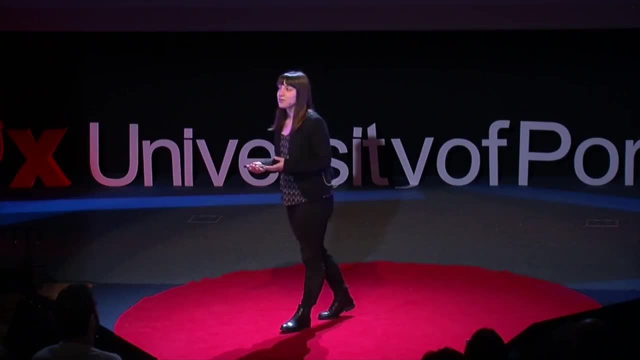 simulate the space radiation, the space vacuum, but we have also done a lot, of, a lot of experiments in situ. so we have sent bacteria and other microorganisms to space, we have put them on the outside of the International Space Station where they are exposed to the real space vacuum and the real space radiation. 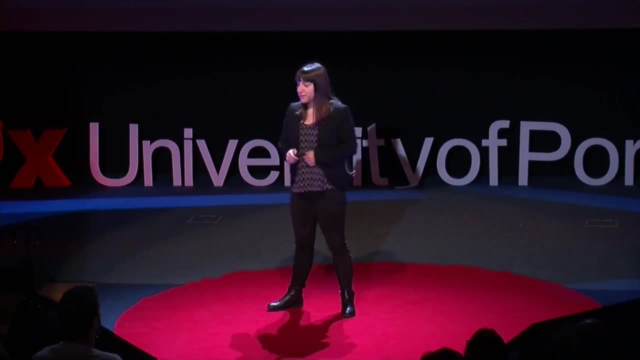 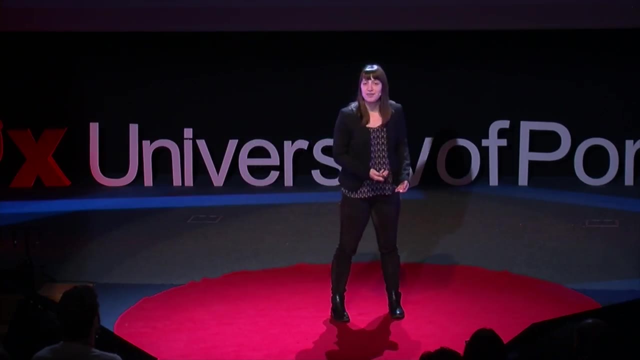 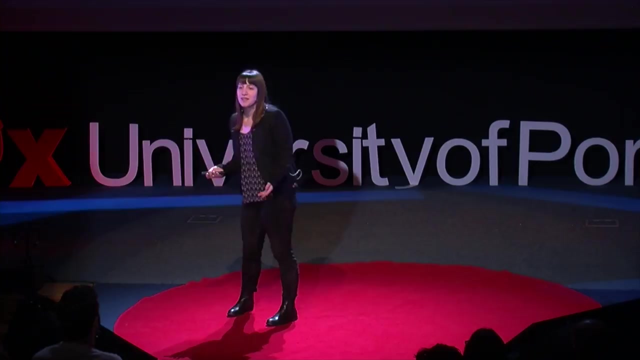 So they stood there for months and what we found out is that many of them actually survive. So this raises the question: if life survives to the extremes of space, where else can it be? What other environments can be habitable? So the first place we actually look, of course, is our own solar system. 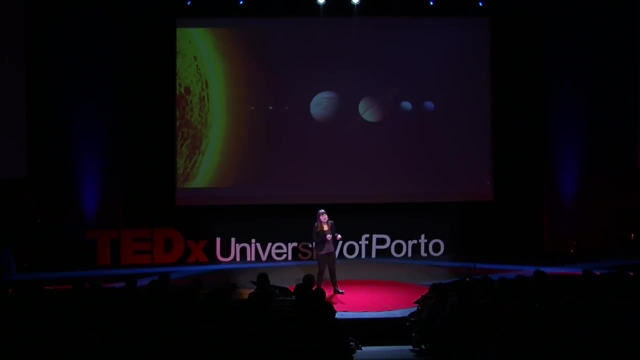 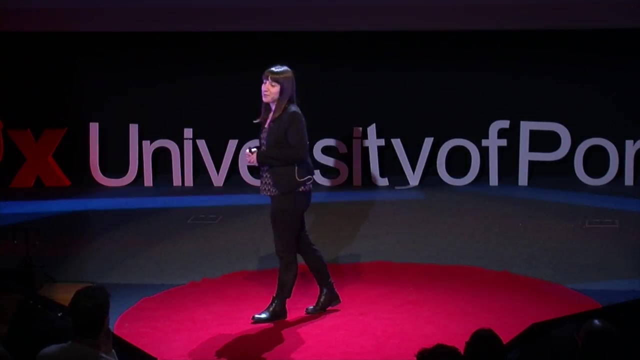 We begin by looking at the Moon. We went there. there is not, it seems there is no life there. But then we focus on other things. Now our second favorite planet is Mars, but also other moons of Jupiter or Saturn are beginning to raise interest. 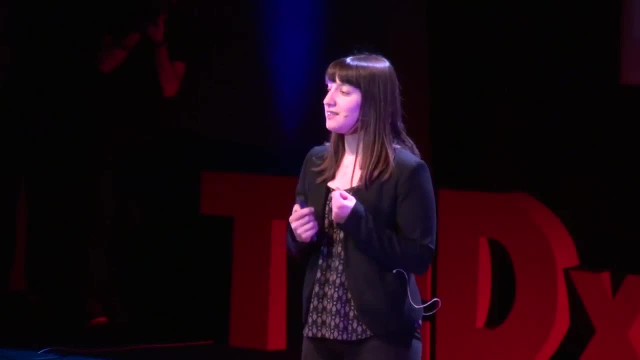 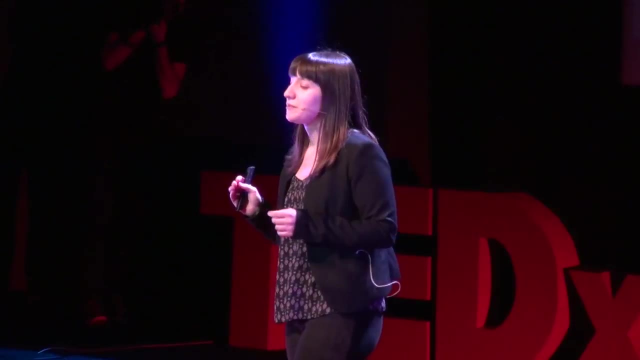 But what really gives astrobiology an interesting twist was the discovery of the first exoplanets. Exoplanets are planets that are outside of our solar system, in other planetary systems. The first one was only found in 1995.. Before that, we had no confirmation that a planet existed outside of our solar system. So after that, with the use of mainly of the Kepler telescope, we discovered a lot more exoplanets. One of the first was actually named Kepler-16, and it became quite famous. but only because it was similar to the planet Tatooine of Star Wars. It had two suns. It looks familiar Now with all of these exoplanets. we can know what other environments are there. We can check for habitable conditions. But there is one- it's one of my favorites- that is right here in our solar system. That is the Jupiter's moon, Europa. Europa is very interesting, but mainly because it has a big ocean. This ocean has about 100 kilometers long.